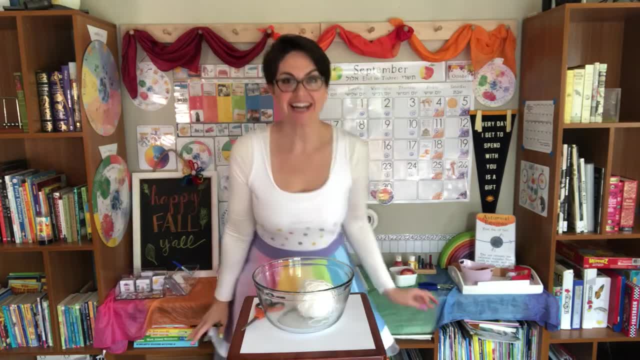 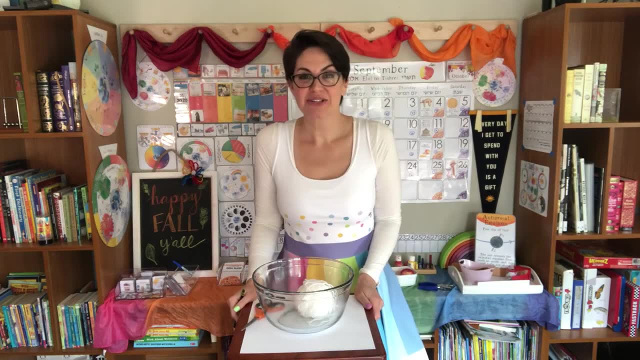 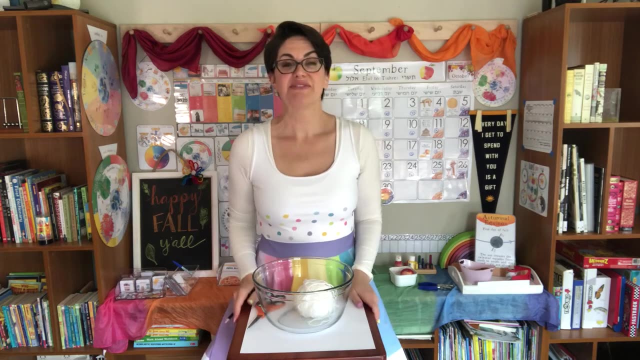 You're here. You are just in time. I thought today we could make a fun craft. What I was thinking of making is something called a phenology wheel. Phenology is the study of nature and how it changes over time, And a phenology wheel is just a way of recording our observations of the natural. 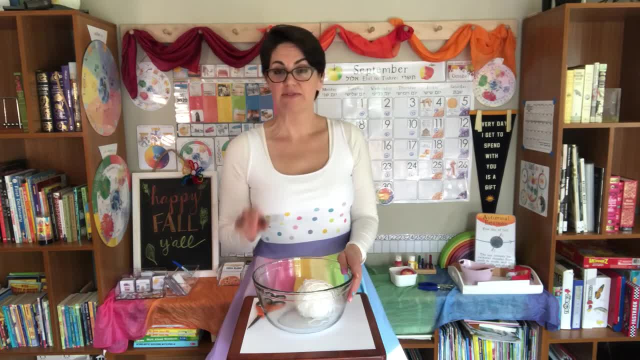 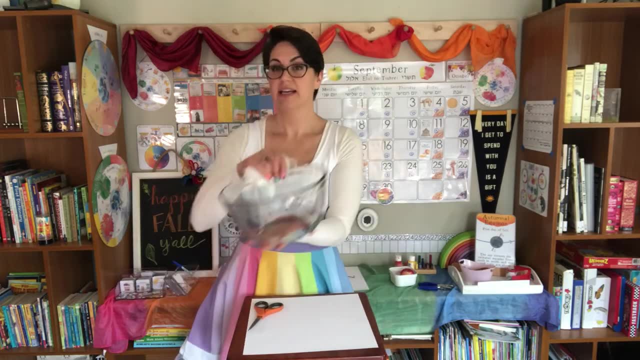 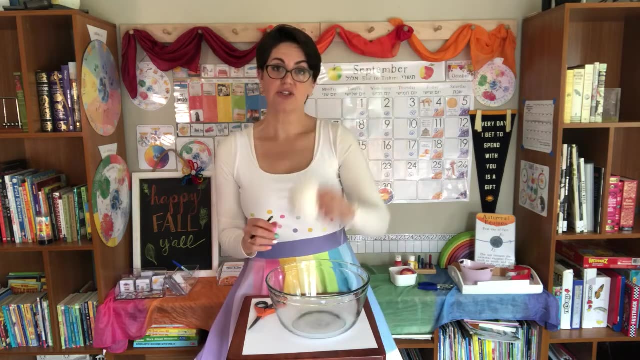 world around us. So to make a phenology wheel is very simple. You will need a piece of paper. I have a big square right here. I'm gonna use a big mixing bowl to make a circle. I'm gonna use some string to show you how to find the center of a circle when you don't have a special tool to do. 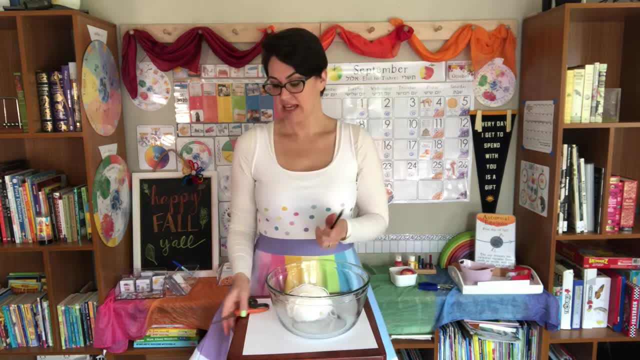 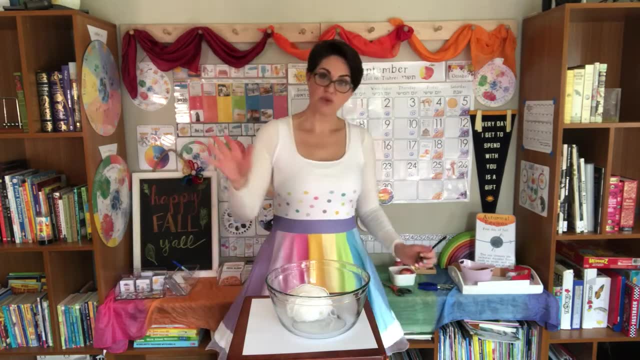 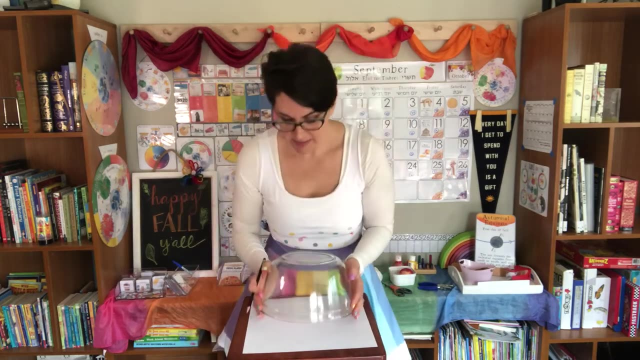 it. I'm gonna use a pencil to trace my bowl and I'm gonna use scissors to cut out my wheel. So here's how we do it. If you need to gather your materials, you can pause the video and go get them now. So I'm gonna take my bowl and put it upside down on my wheel. Now for this phenology wheel. 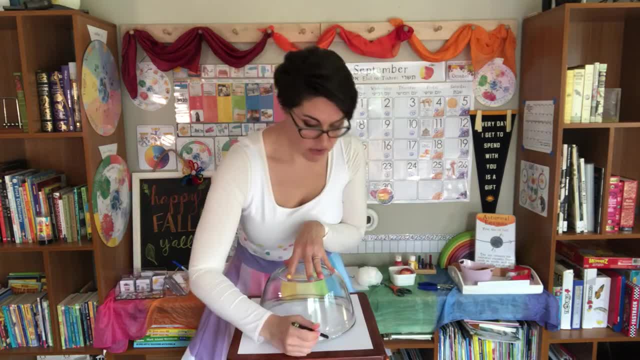 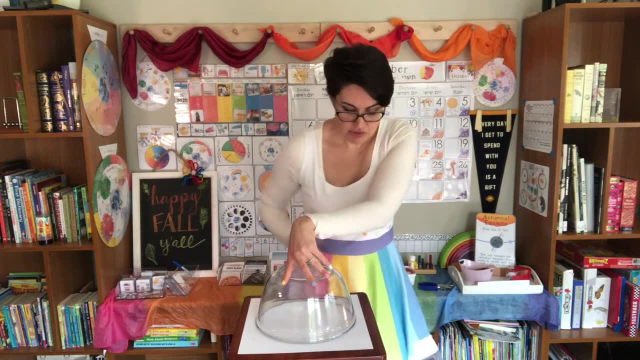 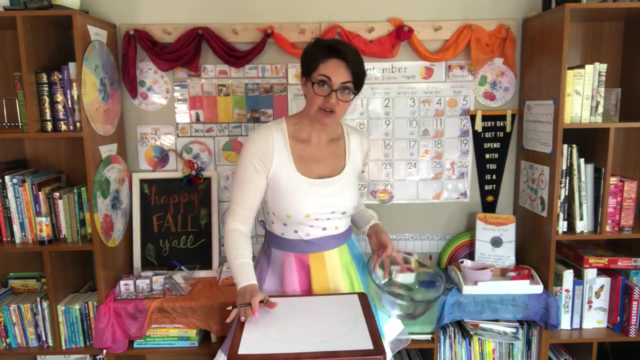 it's best to use paper that's light in color, because you are going to be writing and drawing on your wheel. Once your bowl is upside down, you just trace around it and that gives you a really nice circle. You could draw your own circle too, but I like to use a bowl because then it's really 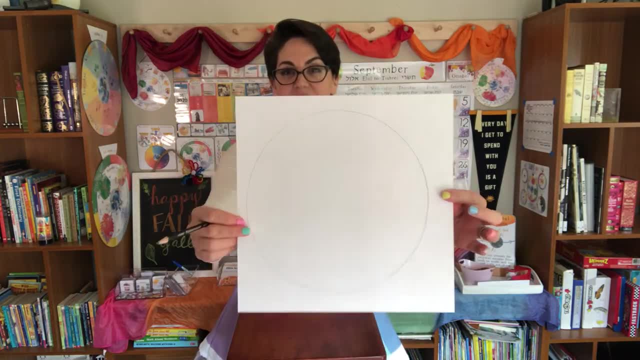 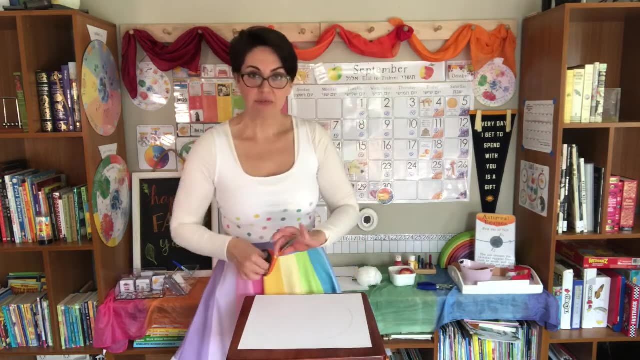 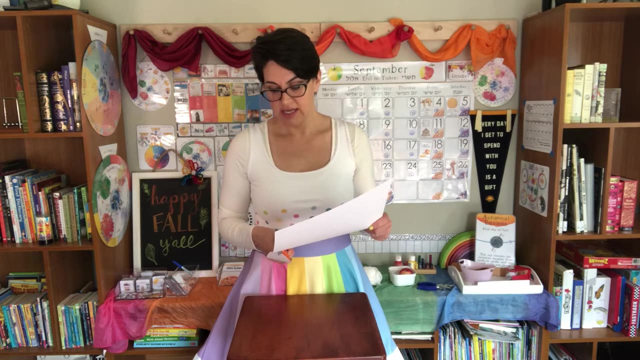 really, really perfect. So here, I don't know if you can see my circle, but now I'm gonna cut it out. So if you need help from your grown-up, you can ask your grown-up to cut your circle or you can do it yourself. Now I think I've told you before that I am not the best cutter of circles. 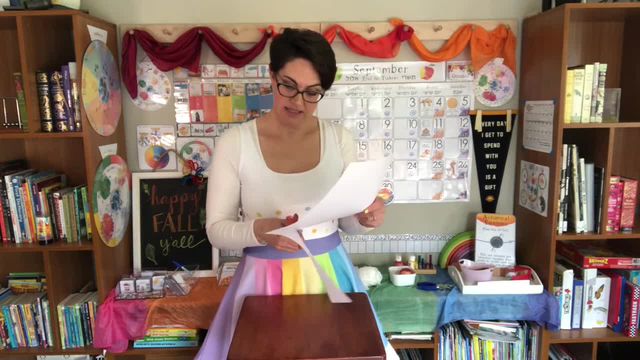 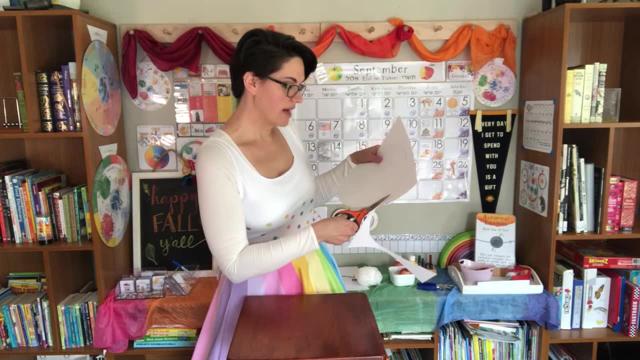 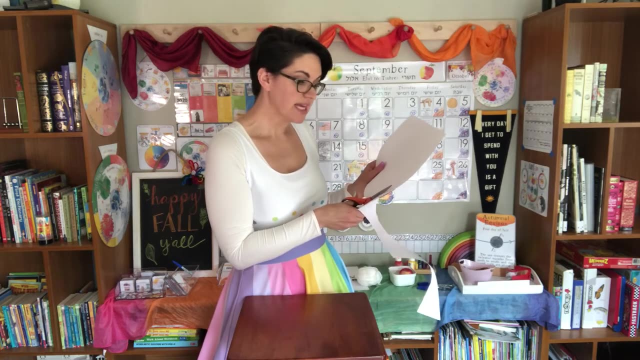 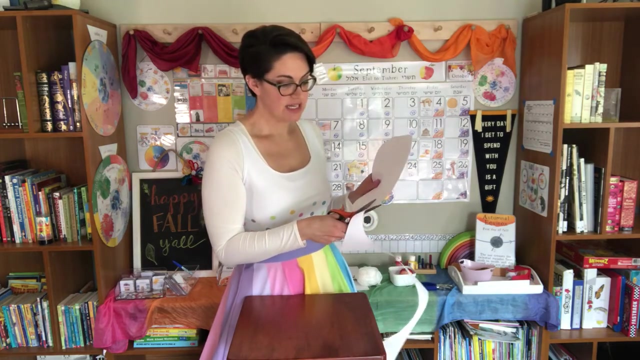 But as long as I'm trying my hardest, that's all that matters. So I'm just cutting along the line that I drew around my bowl, and if your bowl is bigger or smaller than my bowl that doesn't matter, That's okay. As long as your bowl fits on your paper, then it works. The bigger the bowl and the 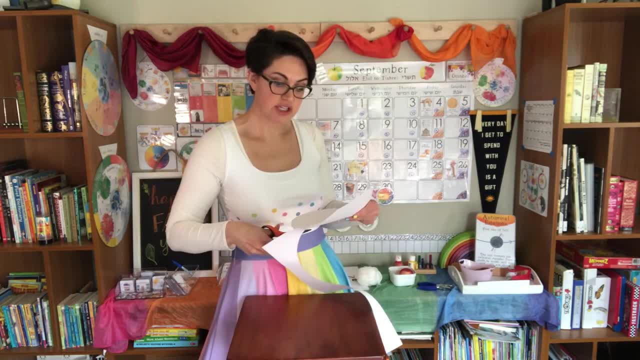 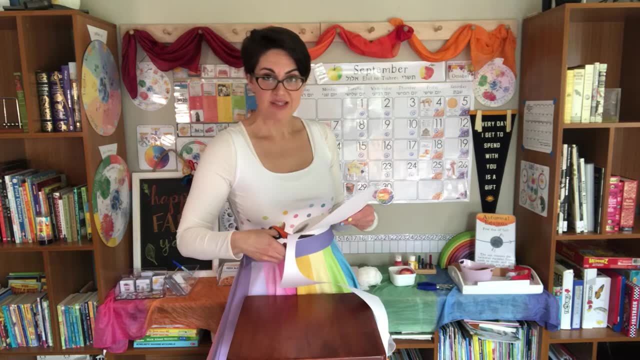 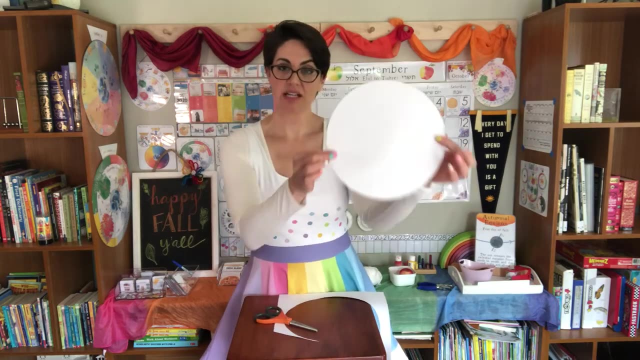 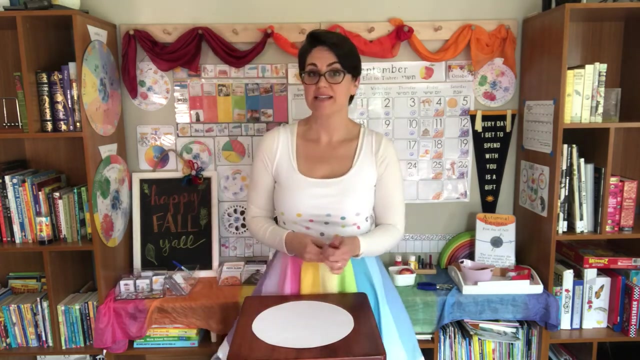 bigger the paper, the more space you'll have to record your paper. So I'm gonna go ahead and cut out my circle. So I'm gonna go ahead and cut out my circle. This is going to be my finology wheel. Now, the reason I decided to make a finology wheel today is because I'm coming to you from a very special day of the year. 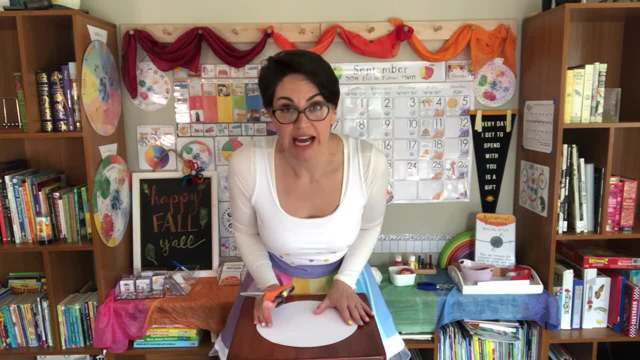 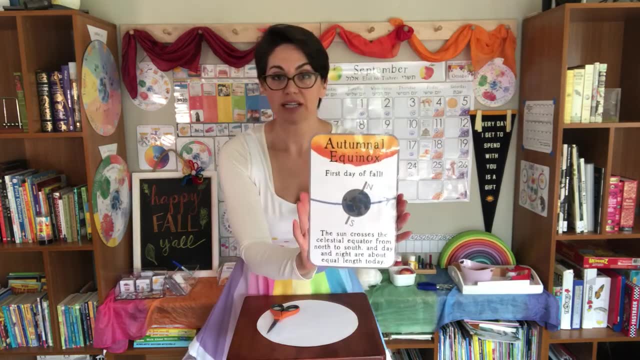 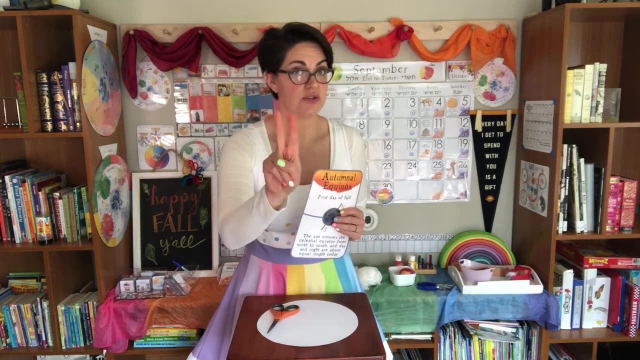 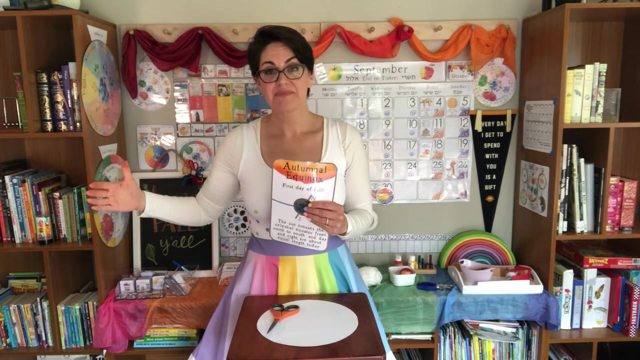 Today is the autumnal equinox. It's the day when the seasons change from summer to fall. It's the first day of fall And since it's an equinox day- there are only two equinoxes a year- I know that today, the daylight part of our day is going to be almost exactly the same length as the darkness part of our day. 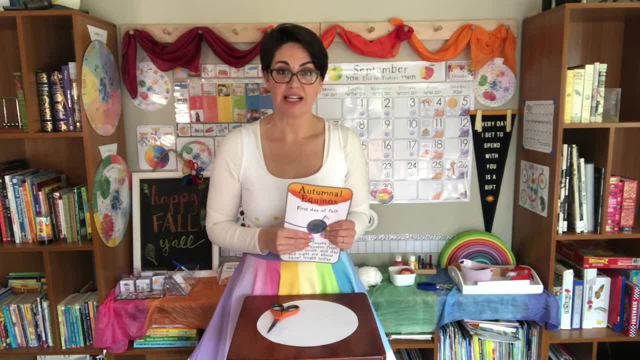 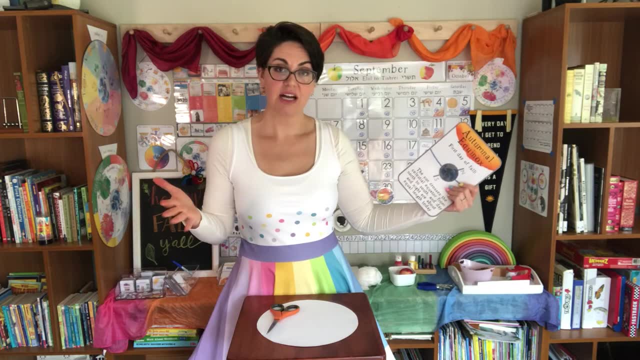 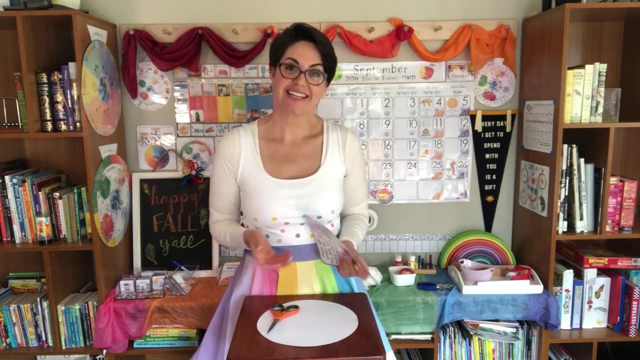 And starting tomorrow with fall, the daylight's going to get shorter and shorter over time and the nighttime is going to get longer all through winter until we come to spring, And then the days will start getting longer again. So you can start a phenology wheel anytime you want. 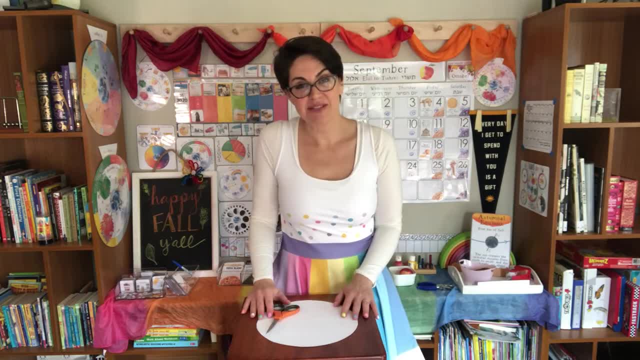 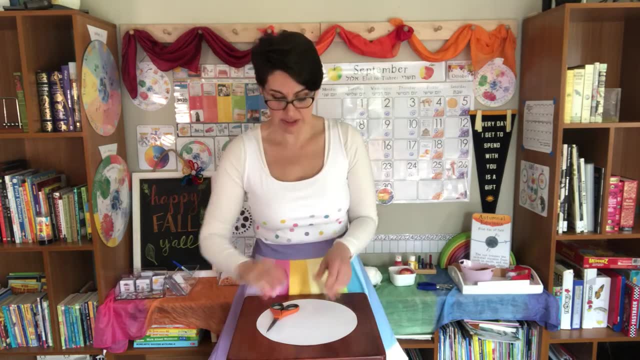 but the change of seasons is a really fun time to do it, because this is when the weather starts to change And this is a really good time to start observing the world around you. So once you have your circle, this is where my handy-dandy string trick comes in. 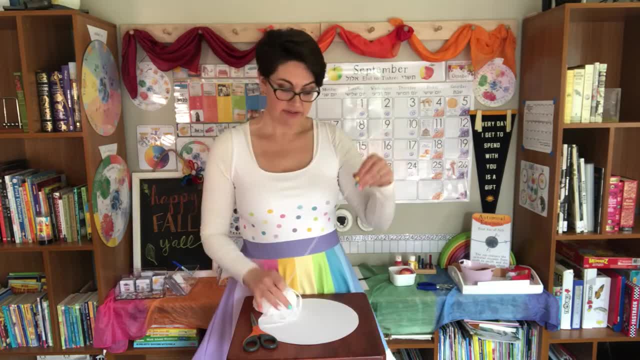 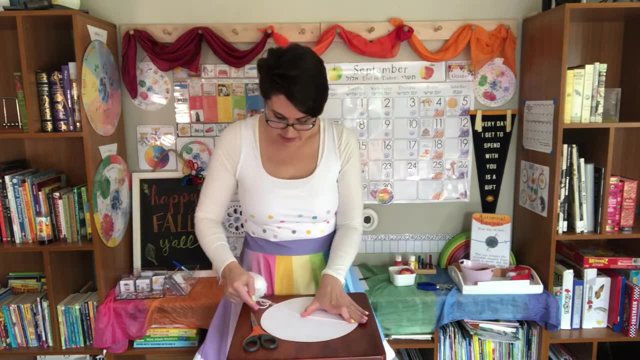 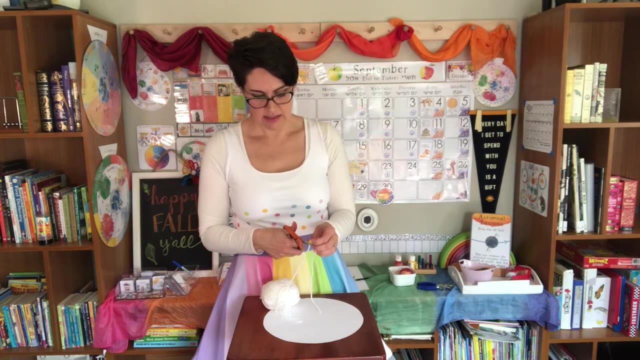 You can take any length of string you have and just measure it, so it's as long as your circle. So I'm putting my string down here and I'm just going to cut it right where my circle ends. Okay, Okay, Okay. 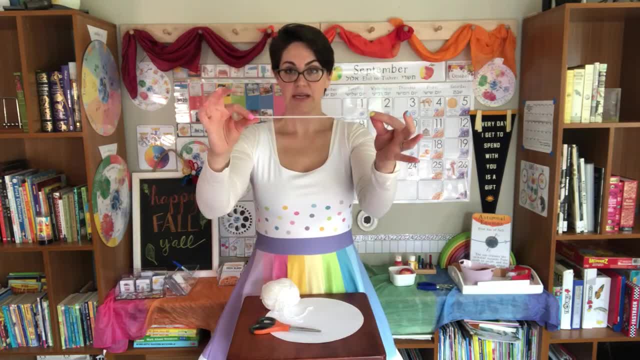 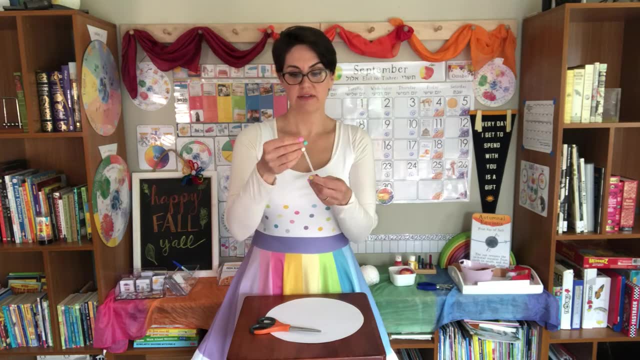 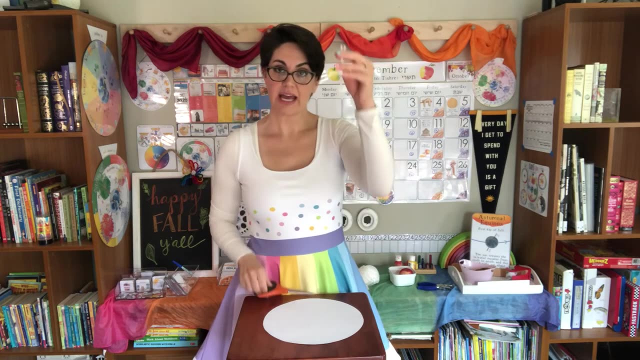 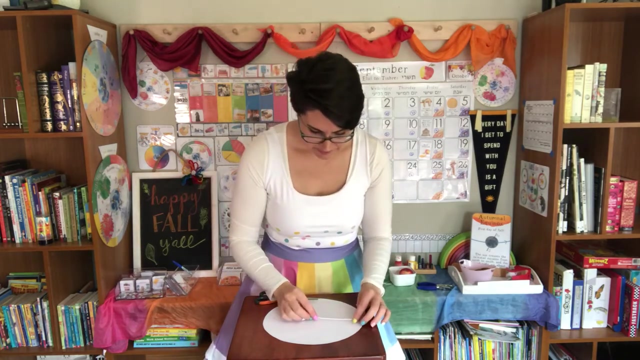 Okay, Okay, This string goes right across my circle, and then I'm going to cut it again in half right, like this, And now the string I have left is going to be half the length of my circle, And so this will give me about the center point. 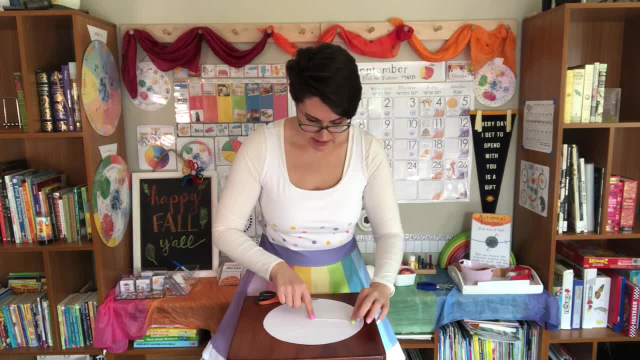 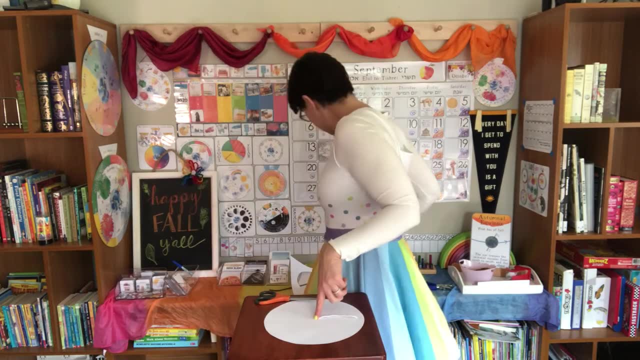 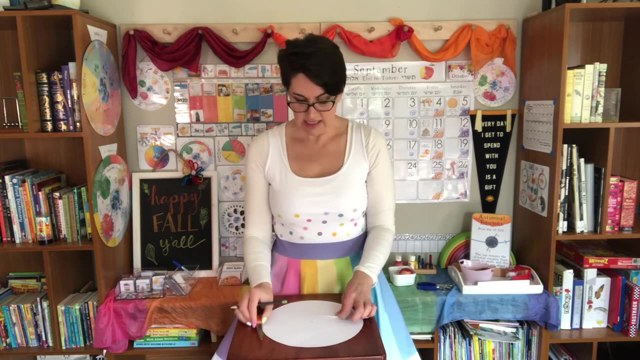 So I'm putting it on top of my circle And I'm going to move it around to see if it looks good And right where that is where the string ends. I'm going to make a dot And it's probably not the exact center of my circle, but it's good enough. 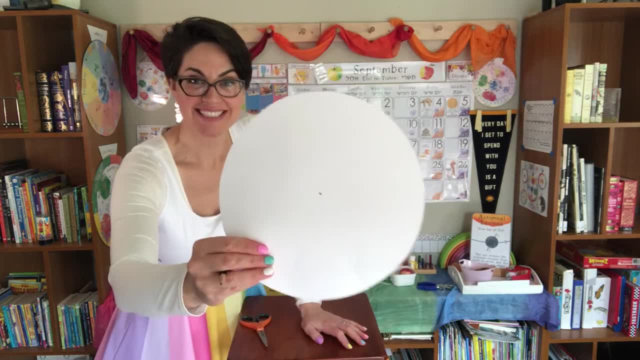 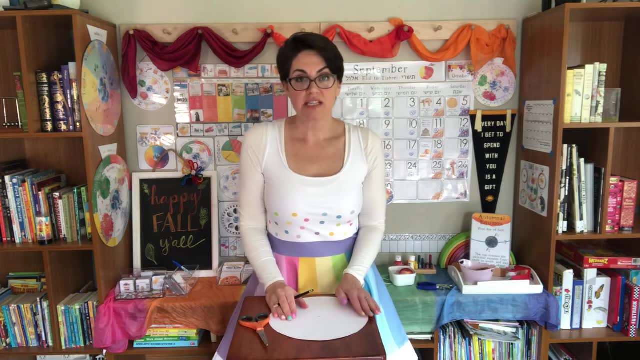 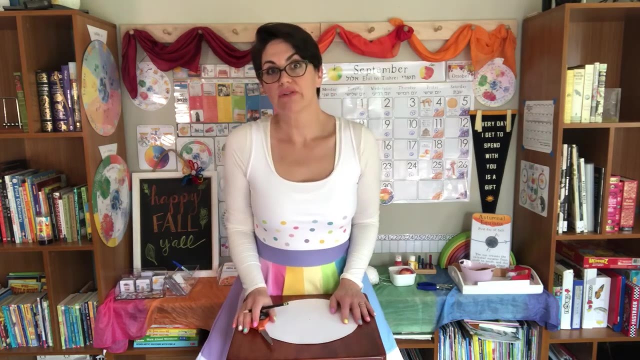 Can you see the dot in the center of my circle? There it is Now to turn this into a phenology wheel. we want to make wedges in our circle, So the easiest way to do it is to make a circle. So the easiest way to do that is to start and make four wedges and then we'll go from there. 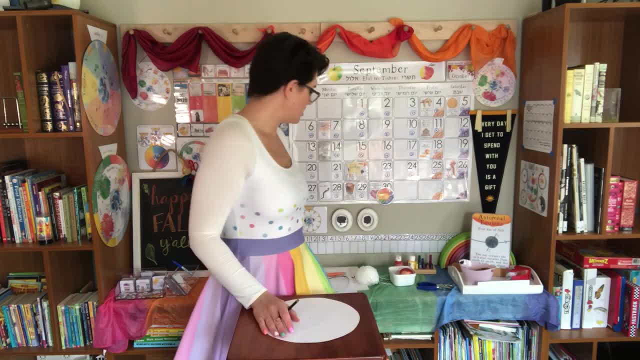 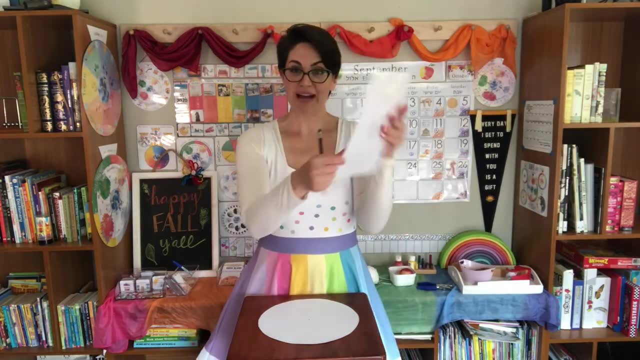 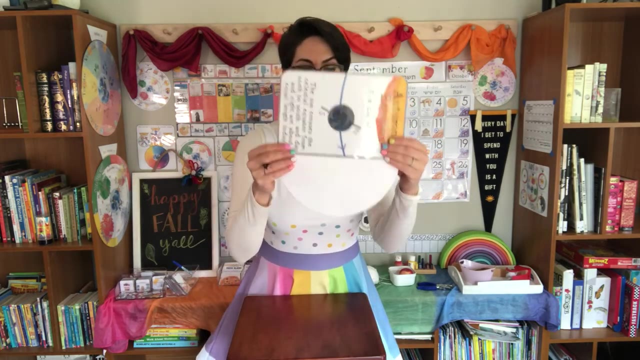 So what could I use to draw a line across my circle? Hmm, You might have a book or anything with a straight edge. I'm going to use my autumnal equinox card. So what I'm going to do now is I'm just going to put it on top of my circle, right above the dot. 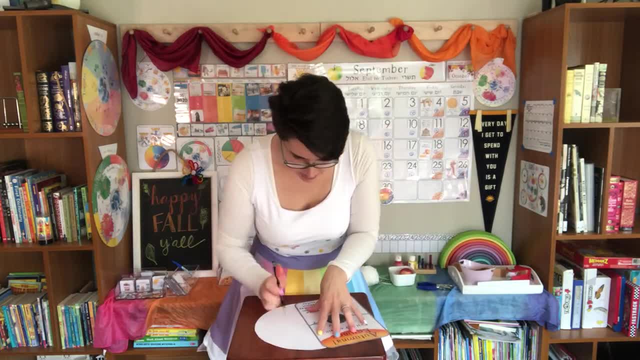 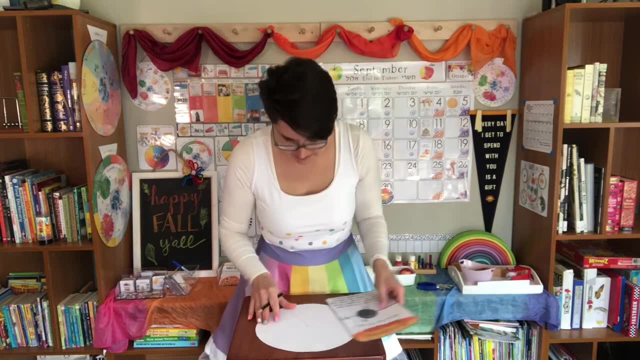 And then I'm going to draw a line, And this isn't quite as long as my circle. Okay, This is my circle, so I have to extend the line past it, but that's okay. Now I have two wedges in my wheel. 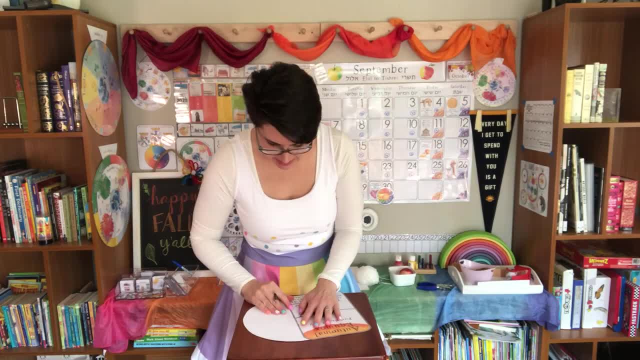 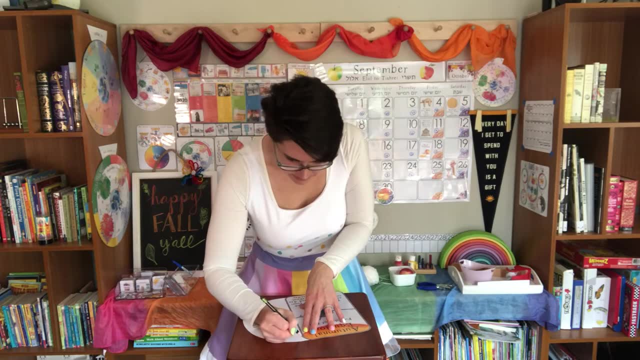 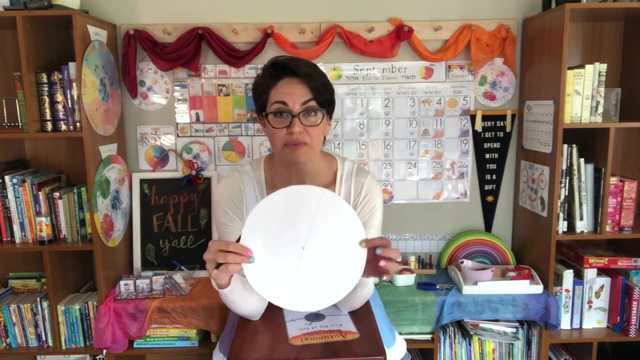 And I'm going to do it again and I'm going to try to make it a 90-degree angle against my first line. And now my wheel has four wedges, So if you want, you can keep your wheel with four wedges. 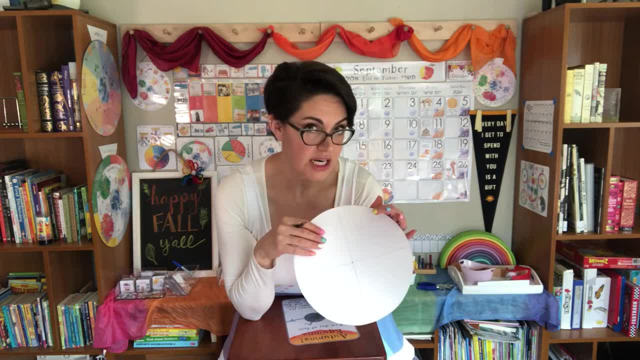 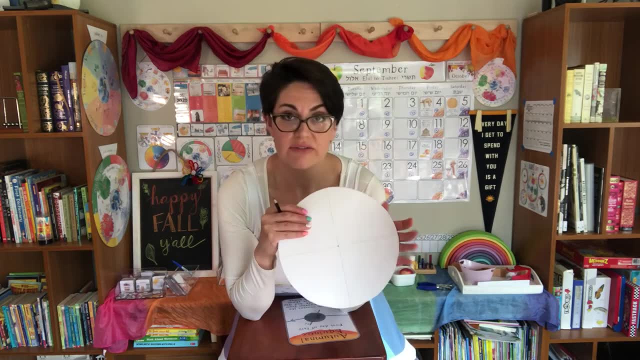 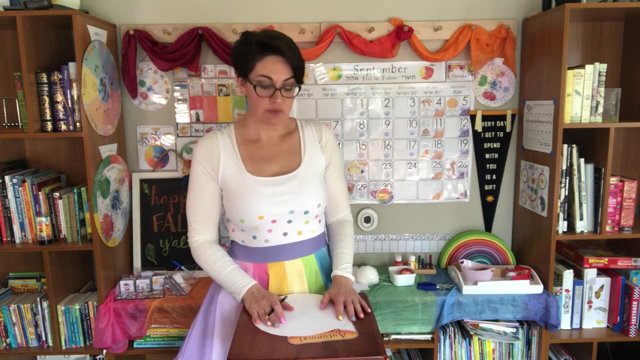 For the four seasons. Or you can give each wheel three separate wedges inside for 12 total wedges, And that will give you the 12 months of the year. I'm going to make mine a monthly phenology wheel, So I'm going to take each wedge and I'm going to draw two more lines in it. 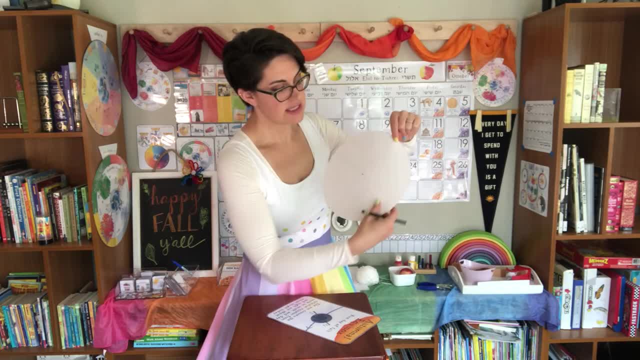 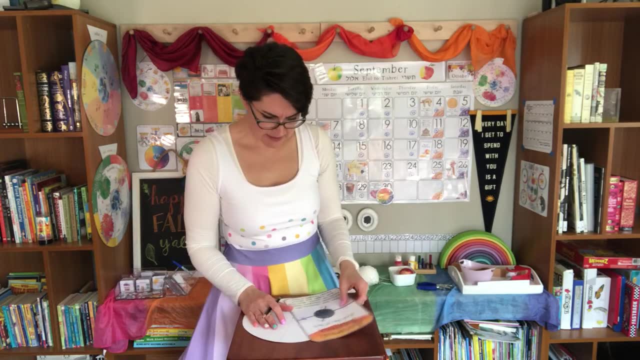 And that will give me three wedges in each quarter for 12 full months. So for this I'm going to draw a line. I'm just kind of guessing because I don't have an exact way to measure what they look like. 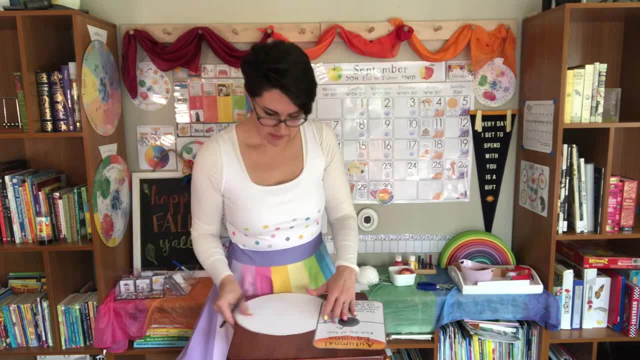 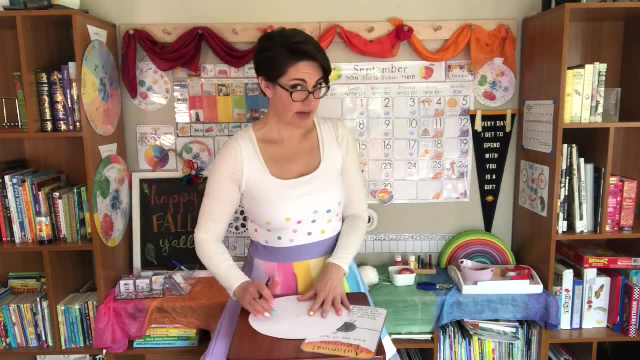 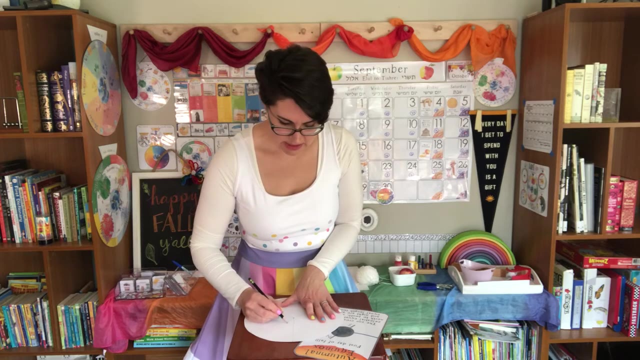 What a third would be. But whatever I do will be just fine. And if you don't want to do any of this drawing on your own- even though I think when you make stuff on your own you like it more- you can download a free phenology wheel from my website. 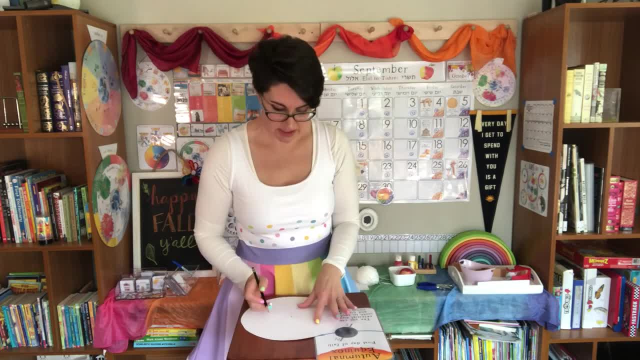 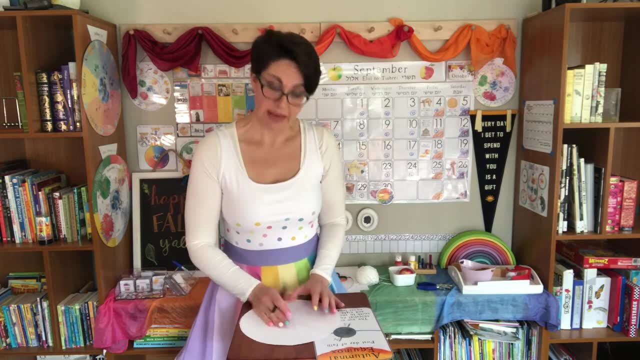 I have a link below for your grown-up to follow And you can just print that out. It'll be an 8-inch phenology wheel, Because that's about as wide as most printers at home will print. So I'm drawing my lines. 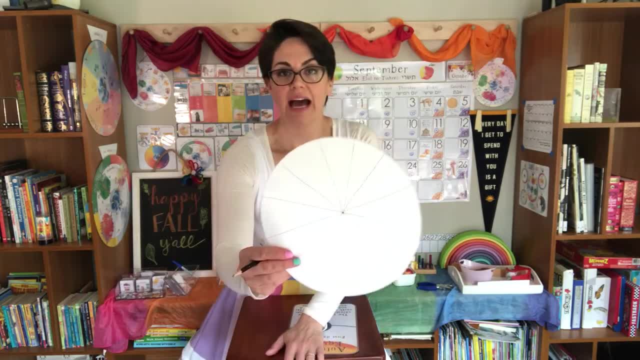 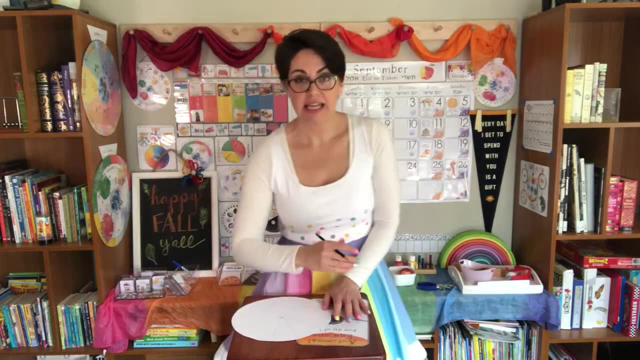 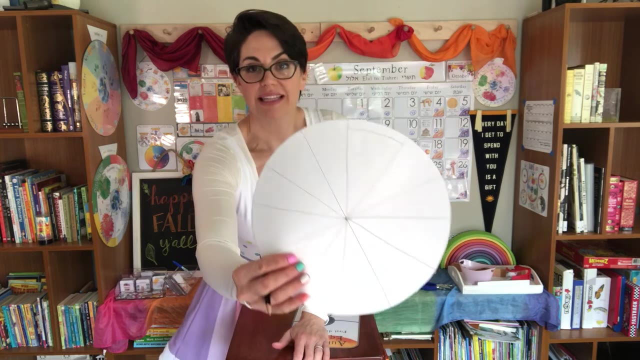 And now I have a circle with 12 wedges. Now I like to do another circle on the outside so I can write the names of the months, And so, if you see, I drew one line at the top of that one wedge. 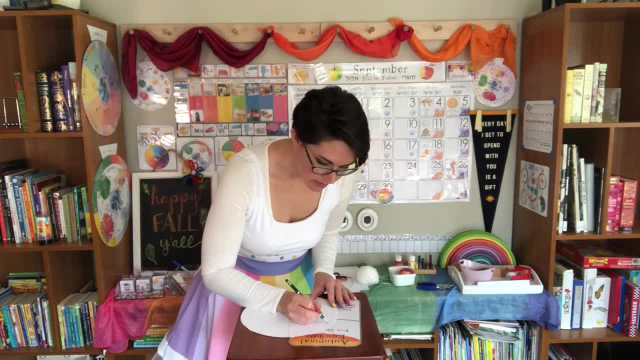 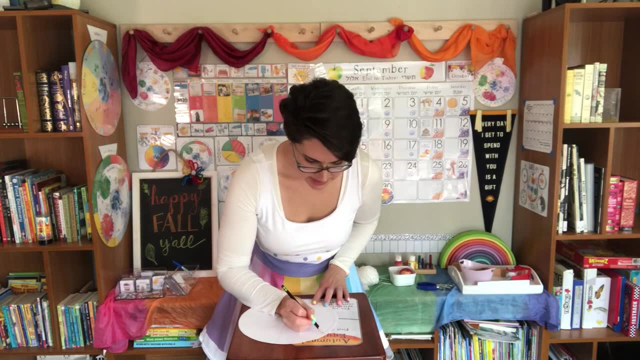 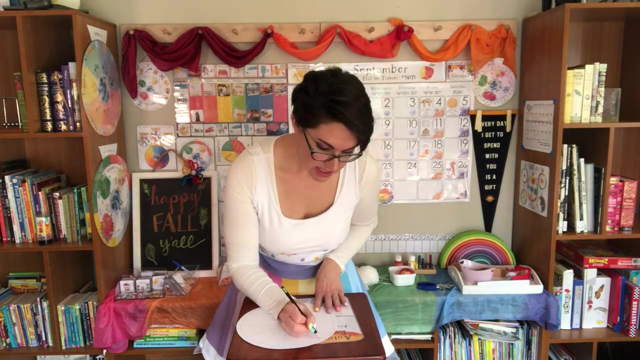 I'm going to do that all the way around my wheel And I'm going to start with September, because that's where we are now. Here we go, And actually I make a lot of round calendars And my round calendars all start with a phenology wheel. 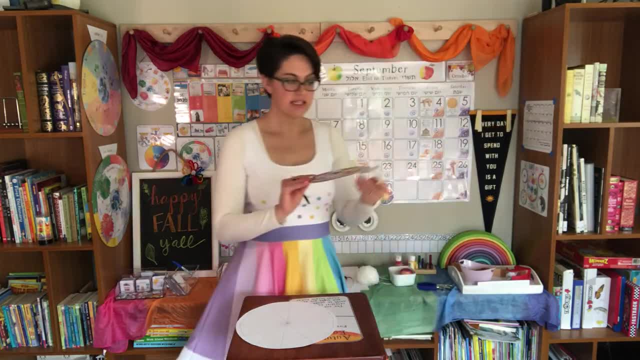 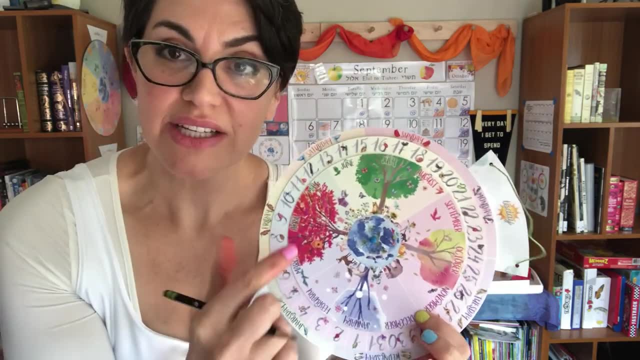 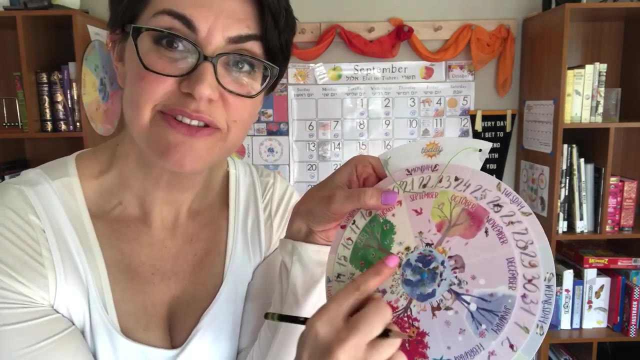 This is my nature season calendar And if you look this, the center of it is a phenology wheel. It shows the changing seasons. And here's today, September 22nd, And the season is turning from summer to fall. 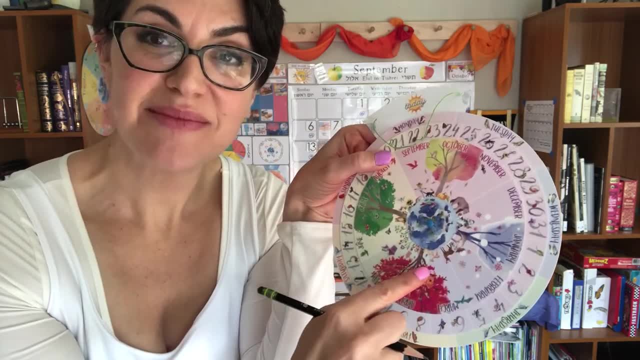 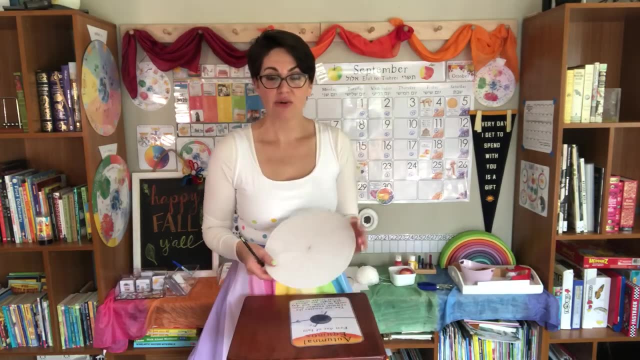 And then it'll turn to winter, And then it'll come to spring And right back to summer For you to make your own phenology wheel. that is so special. So now that I have the basics down, I could take a pen or a marker. 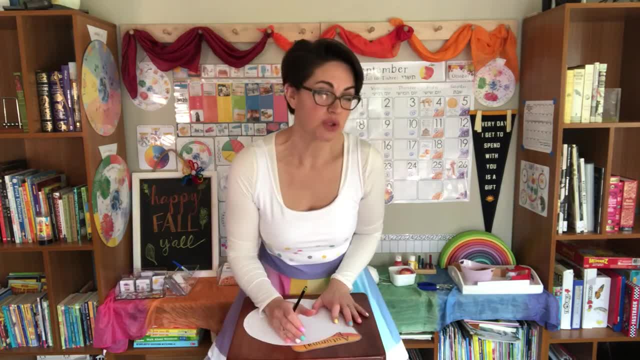 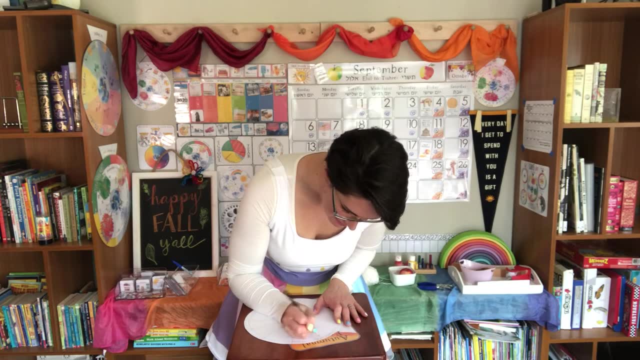 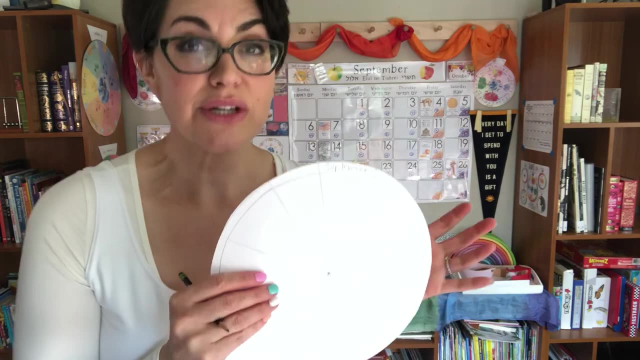 and I could write September. I'm going to do it with my pencil first, just to make sure it looks nice. So I wrote September And now I'm going to take some time to go outside and observe what I see in the world around me.